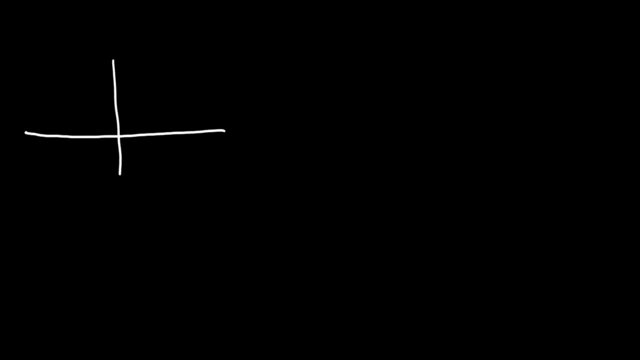 Now in this lesson we're going to focus on graphing quadratic functions used in transformations. So let's start with the parent function. y equals x squared. This graph has a shape of a? u and it opens upward. It looks like that: 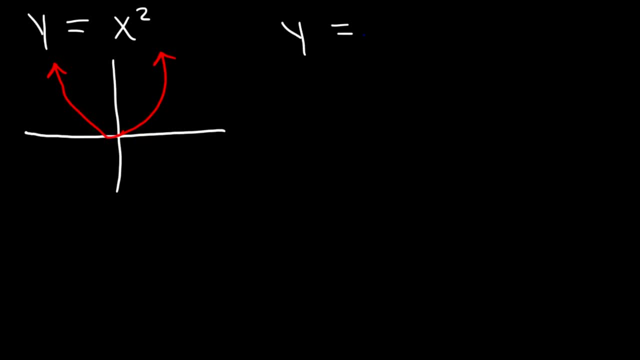 Now what do you think is going to happen if we put a negative sign in front of it? The graph negative x squared, it looks very similar to the first one, but it's going to reflect over the x axis, Which means it's going to face downward instead of opening upward. 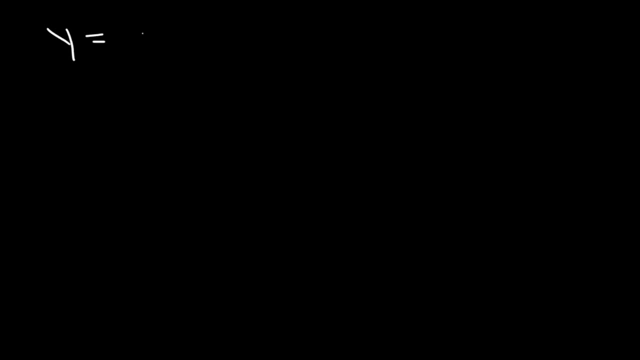 Now what about the graph y equals x squared plus 2?? What effect will the plus 2 have on the graph? Plus 2 will cause it to shift two units upward. So it's going to start at y equals 2, and then it's going to open upward. 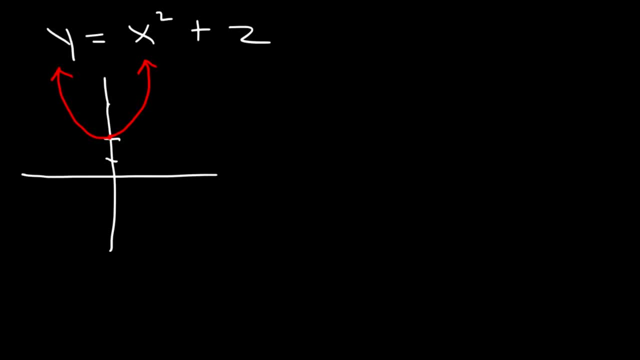 So that's the shape for that graph. Let's say, if we have a negative x squared minus 1.. Minus 1 is the vertical shift, so it shifts down one unit. So it's going to start at negative 1, and because there's a negative in front of the x squared, it's going to open downward. 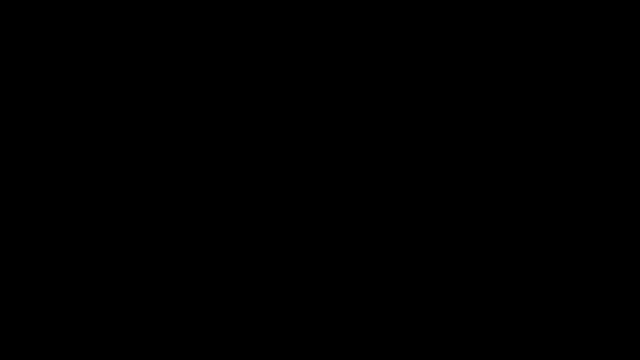 So it looks like that. Now, what about this one? y is equal to x minus 1 squared. This graph is going to shift One unit to the right. If you're ever unsure about this, set the inside equal to 0.. 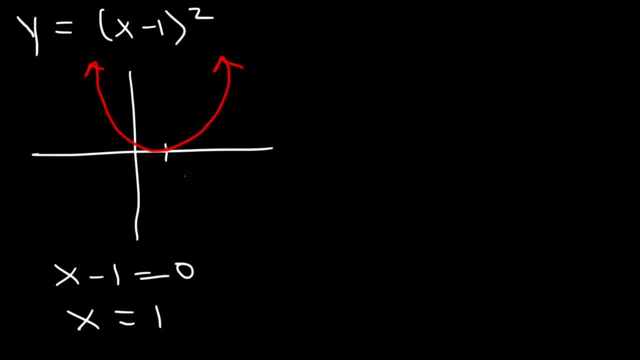 And you'll see that x is equal to 1.. That's going to be the location of the new origin or the vertex. Now let's say, if we have x plus 2 squared, This one is going to shift two units to the left. 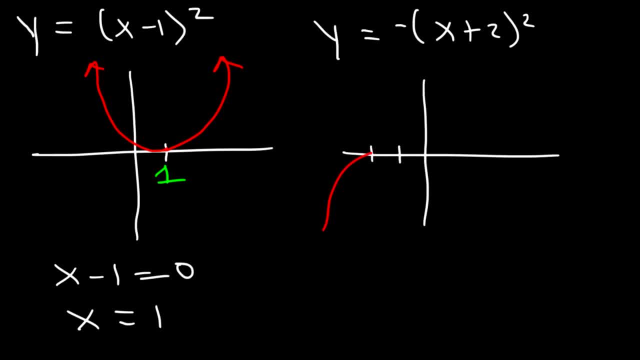 But let's put a negative sign in front of it, So it's going to open Downward. Try these two examples: y equals x minus 3 squared plus 2.. With a negative in front. And then x plus 2 squared minus 4.. 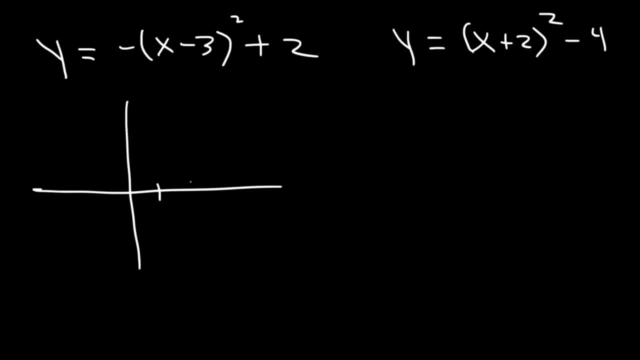 So the first one: it's going to shift three units to the right And up two units. So that's the location of the vertex. The vertex is 3 comma 2. And because of the negative sign, it's going to open downward. 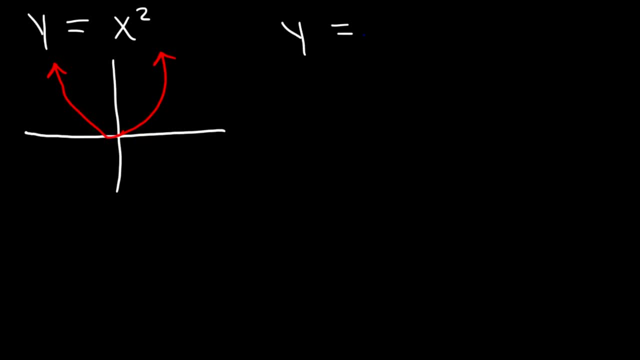 Now what do you think is going to happen if we put a negative sign in front of it? The graph negative x squared, it looks very similar to the first one, but it's going to reflect over the x axis, Which means it's going to face downward instead of opening upward. 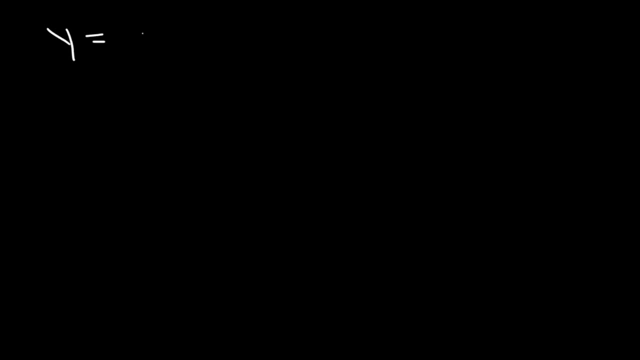 Now what about the graph y equals x squared plus 2?? What effect will the plus 2 have on the graph? Plus 2 will cause it to shift two units upward. So it's going to start at y equals 2, and then it's going to open upward. 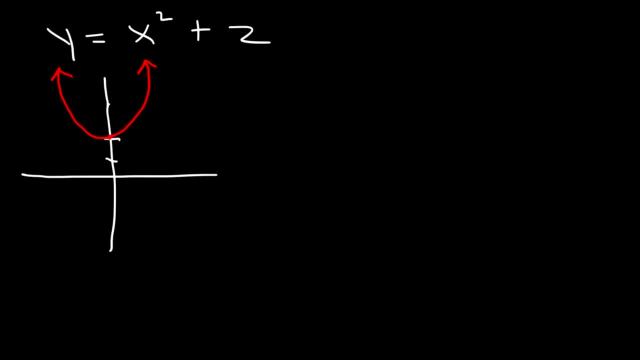 So that's the shape for that graph. Let's say, if we have a negative x squared minus 1.. Minus 1 is the vertical shift, so it shifts down one unit. So it's going to start at negative 1, and because there's a negative in front of the x squared, it's going to open downward. 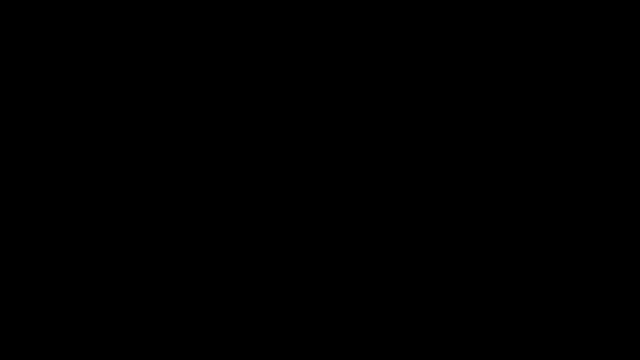 So it looks like that. Now, what about this one? y is equal to x minus 1 squared. This graph is going to shift One unit to the right. If you're ever unsure about this, set the inside equal to 0.. 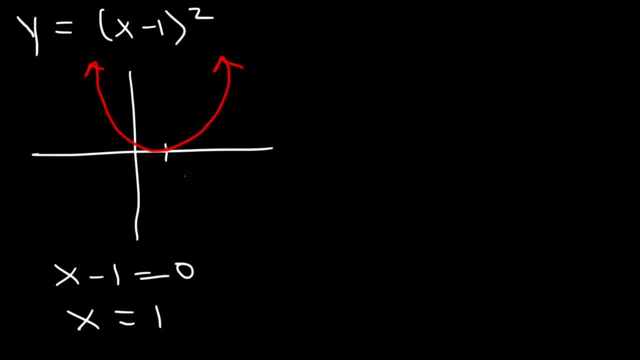 And you'll see that x is equal to 1.. That's going to be the location of the new origin or the vertex. Now let's say, if we have x plus 2 squared, This one is going to shift two units to the left. 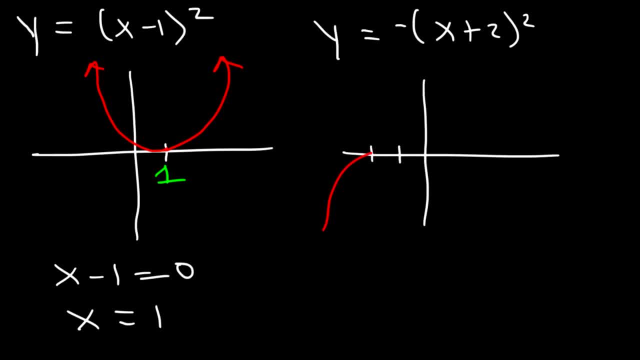 But let's put a negative sign in front of it, So it's going to open Downward. Try these two examples: y equals x minus 3 squared plus 2.. With a negative in front. And then x plus 2 squared minus 4.. 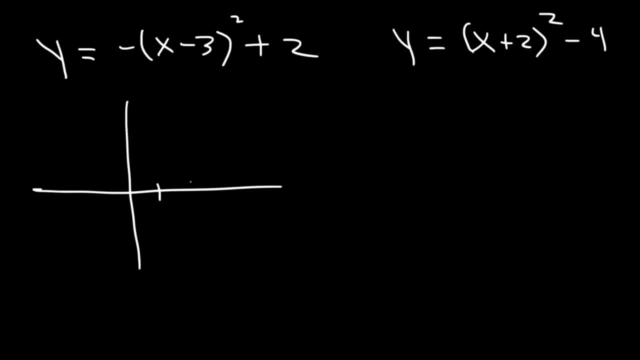 So the first one: it's going to shift three units to the right And up two units. So that's the location of the vertex. The vertex is 3 comma 2. And because of the negative sign, it's going to open downward. 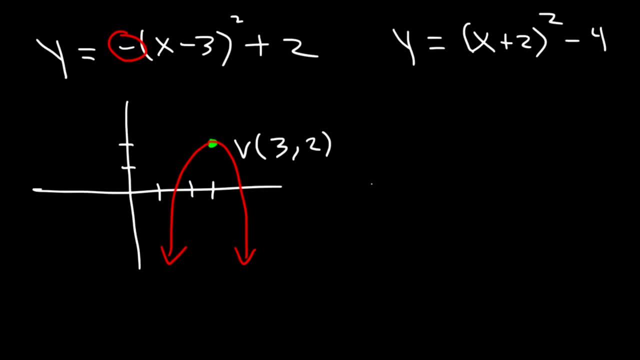 So it looks something like that, And for the last one the vertex is negative 2, negative 4.. The graph shifts two units to the left And down four units, But we have a positive in front of the x plus 2 squared. 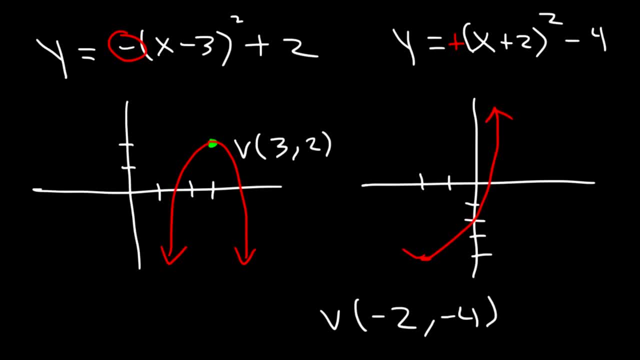 So it's going to open Upward. Anytime you have a positive x squared, it opens upward. If there's a negative in front of the x squared, it's going to open downward. Thank you. 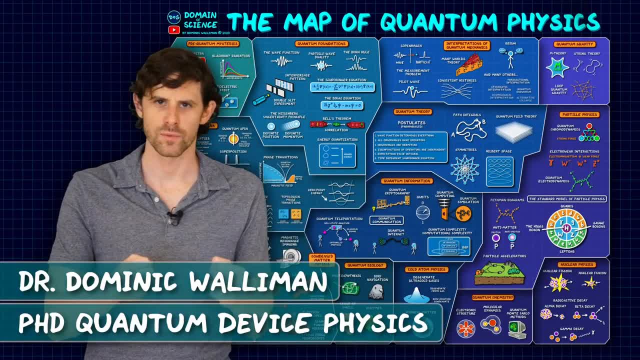 I've been fascinated with quantum physics for a very long time, so much so I did a PhD in it, and I wanted to share the subject with you. So I made this map of quantum physics to lay out the ideas within the subject, to set some bounds on it, so you know it's not endless. 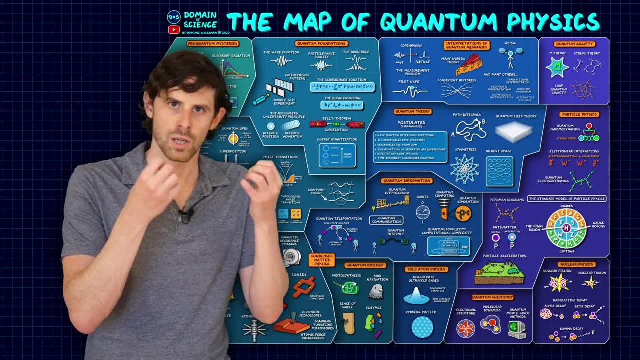 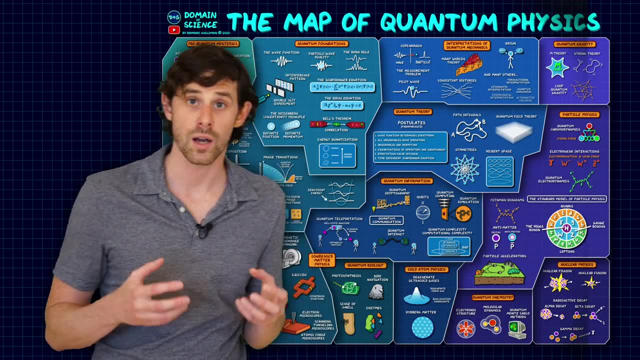 and to introduce you to lots of concepts. If you're interested in them, you can. you can dig deeper. When you're approaching a subject like this that's so complicated, it can be quite challenging because you don't know where to start and you don't know how all the concepts relate to. 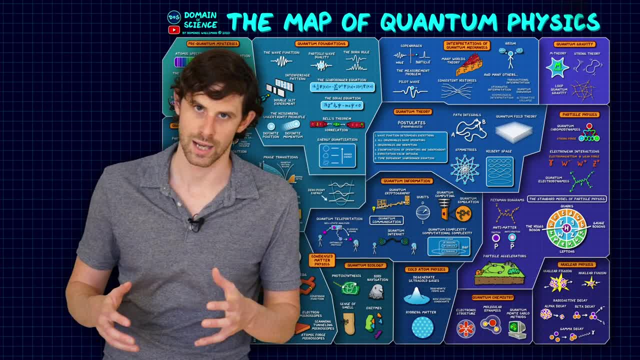 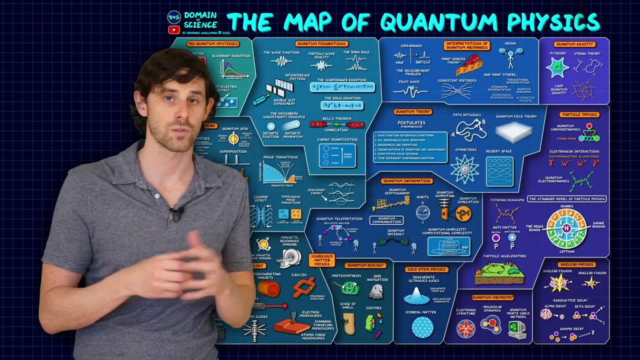 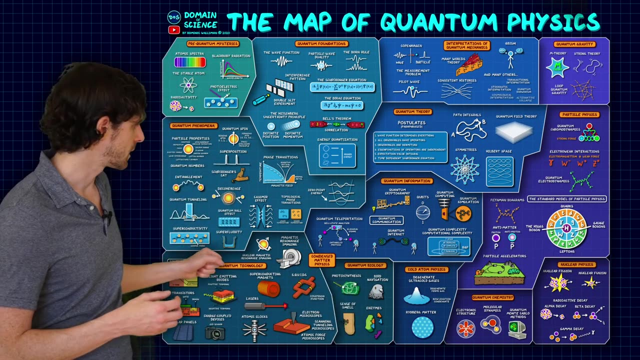 each other. So hopefully this will put everything in context. Okay, first let's just look at the geography of this map. To the north west we have the foundations of quantum physics, and then further south we go through quantum phenomena to quantum technology, And in the south and east we 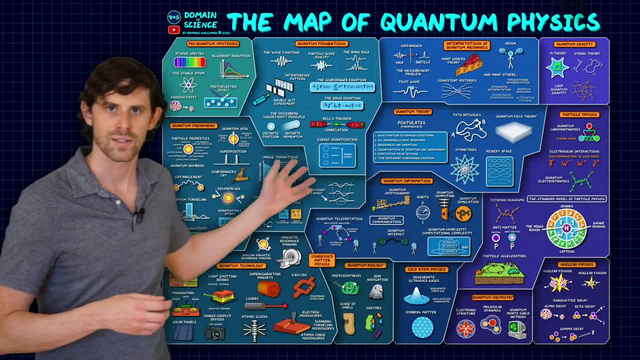 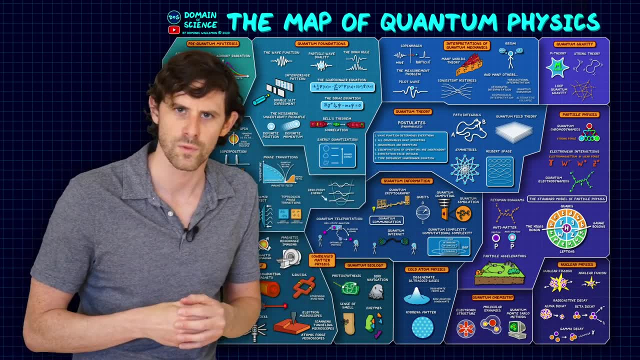 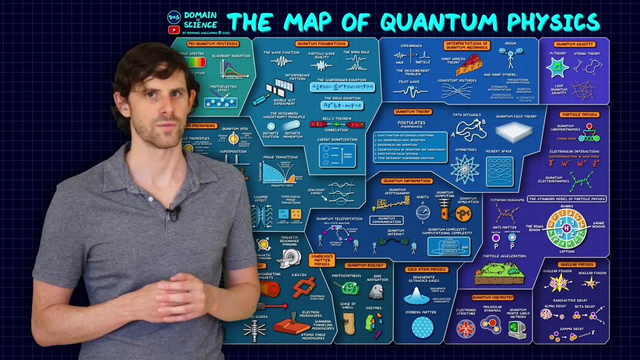 have the academic disciplines of quantum physics- In the centre quantum theory, and in the north and east the theoretical future of quantum physics beyond what we already know. That is your quantum forecast for this video. I've also made a poster of this available, so if that's of interest, check.